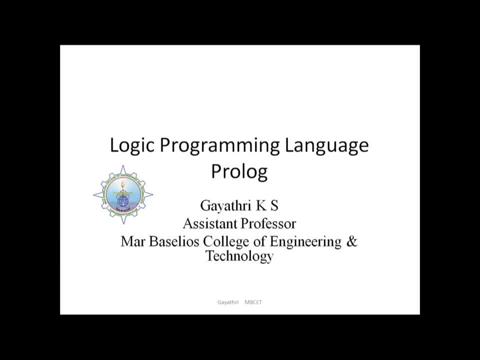 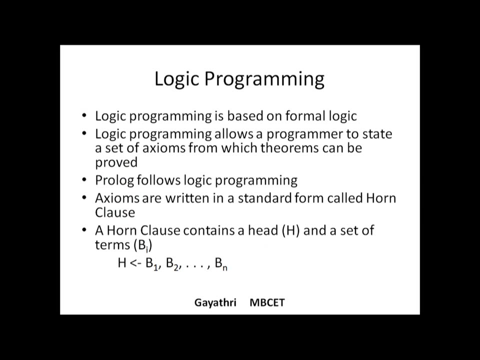 Hello all, Welcome to my next lecture series on logic programming language. So I will be explaining about Prologue in a couple of lectures. So before going on with Prologue, we will see what is a logic programming. So logic programming is based on the formal logic. 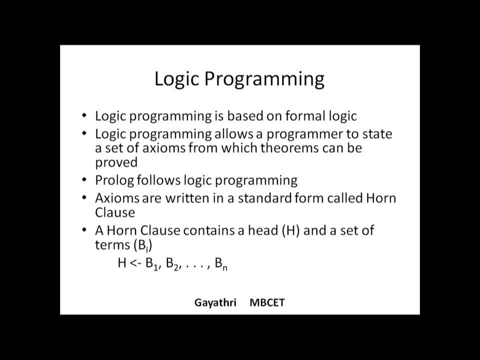 It is based on the logic. So logic programming allows a programmer to state a set of axioms from which we prove theorems. So we will be providing set of axioms from which we prove theorems. That is logic programming, Prologue. it follows logic programming. So we have to state a. 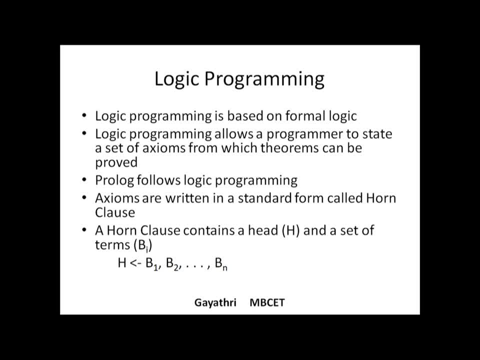 set of axioms and from which we can derive theorems. So the axioms are written in a standard format called Horn Clause. Okay, So axioms are written using Horn Clauses. So we should know what is a Horn Clause, A Horn? 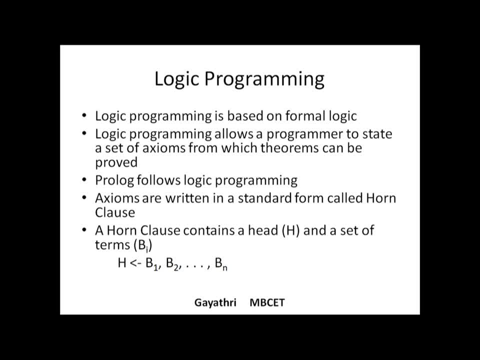 Clause. it contains two parts. One is the head H and the other one is the set of terms denoted by B, I And the Horn. Clause is written like: this Head implies the different terms: Okay, This symbol indicates implies, and this comma indicates and. 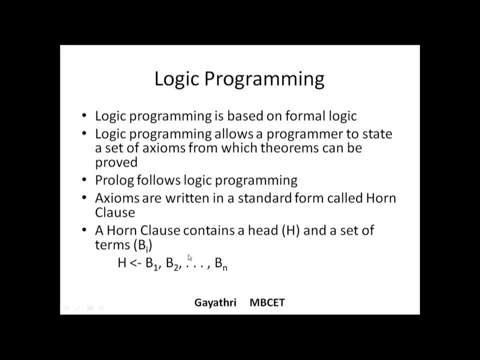 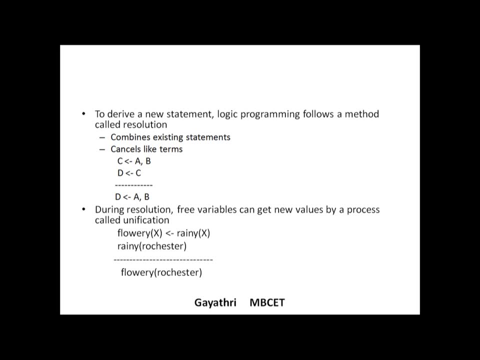 So each and every B are called as terms. Okay, So this is the head and these are the terms. So there are N terms. The terms are linked using AND operator. We will see an example. So to derive a new statement, logic programming follows a method called resolution. Okay, We will look into detail. 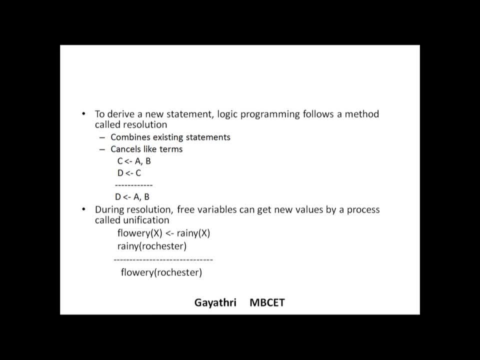 what is resolution? and all for now, just to know the concept. So, logic programming: it follows a method called resolution to derive a new statement. Okay, So this resolution, how it works, is from the given statements. it combines the existing statements. Okay, It combines the. 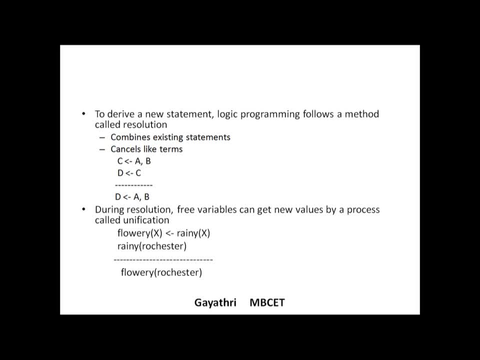 existing statements and it cancels out like terms. Finally, whatever is resulting is the new statement derived from the existing one And the entire process is called as resolution. Okay, So resolution means it involves two steps. First, one is combines existing statements and, after combining it, cancels the like terms. Whatever, 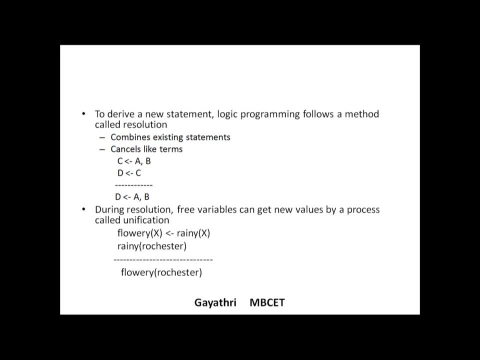 resulting is the final derived statement And the process is called as resolution. Now, during this resolution process, if any free variables are there, they will get values by a process called as unification. So when you are doing resolution, if there are any free variables, they will be associated with. 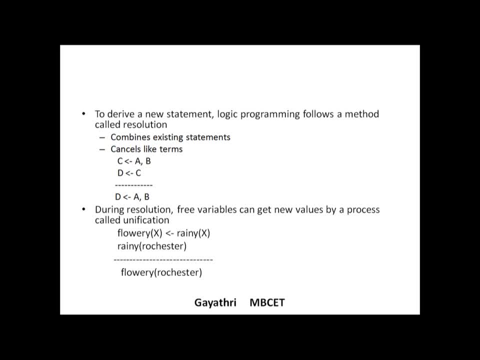 some values as part of this resolution and the process is called as unification. okay, so, uh, example of resolution is here. i have two horn classes, uh, a comma a and b implies c and c implies d. so i'm combining these two existing terms, okay, and i am canceling, like. 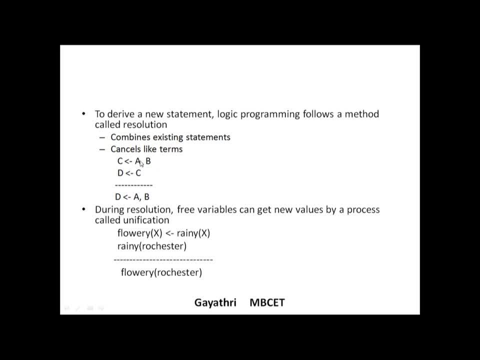 terms. so c will be cancelled, which gives me like a and b together implies b. so this is the result of unification. sorry, this is the result of resolution. okay, so we will see what is unification. so unification means you are giving values to variables. okay, so now i have a horn class like 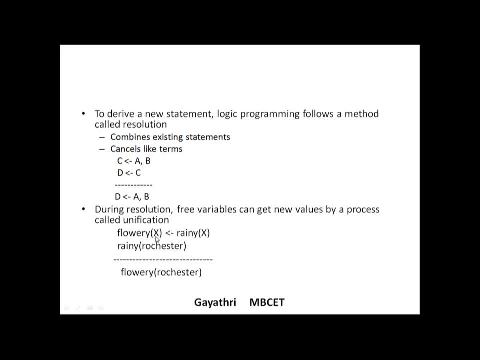 rainy of x implies flowery of x and rainy of rochester, only the head part of the Neighbourhood. Х implies flowery of X, so i'm taking the values of my share also. is there? there is no term. okay, rainy of rochester. now, here you can see. there is only a single free. 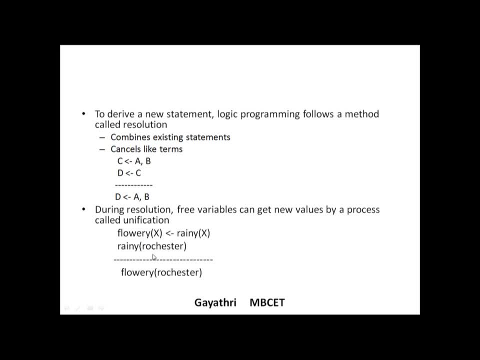 variable x, okay, and here you have some values. so, as part of this unification- unification, sorry, resolution- means combining these two together and cancelling out like terms. so these two will be combined and rainy of x will be cancelled. finally, this plovery of x is remaining and this: 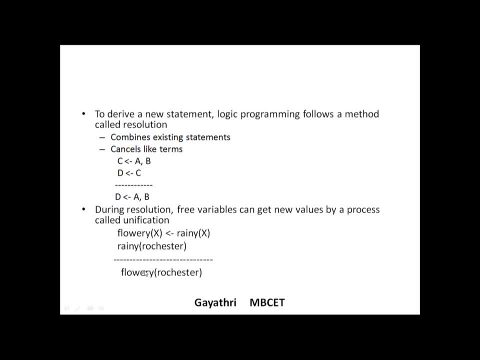 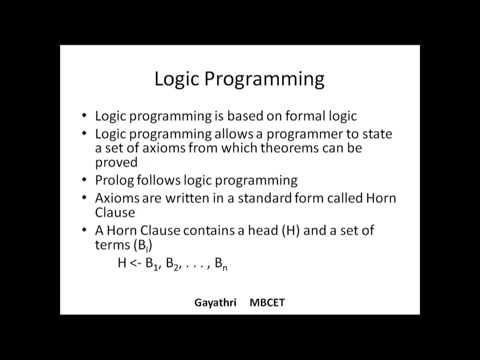 x will get value from this rochester, so we will get the result as plovery of rochester, which is obtained as using both resolution as well as unification. okay, so only this. this much introduction is needed for logic programming. so logic programming it is basically, i mean, standing on logic. okay, so logic, how you have. 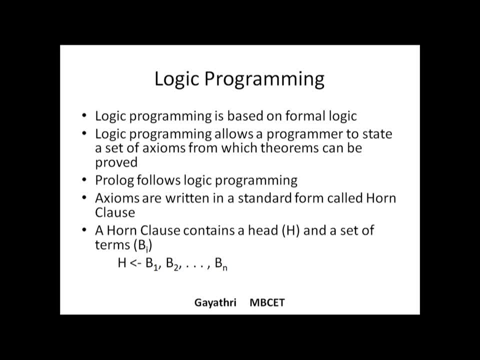 to provide us. you will provide a set of axioms from which theorems can be proved. Prologue is an example of logic programming. So this axioms need to be provided, which will be provided in a standard form called Horn class. Horn class has two parts: one is the head and the other one is 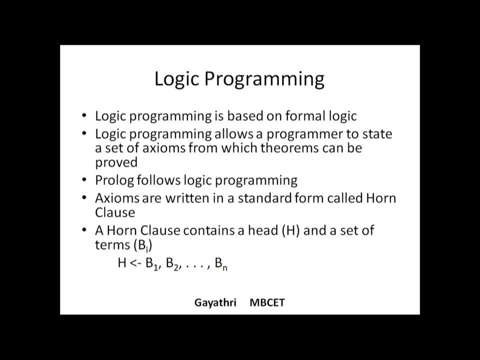 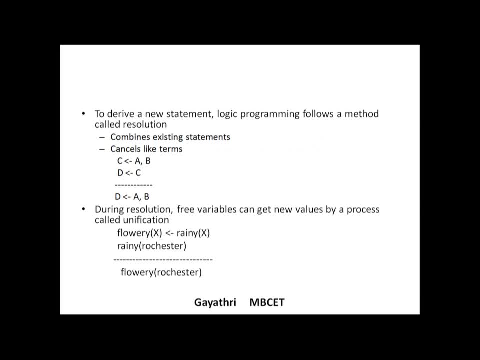 the list of terms, and these are head. and terms are connected using implication and terms are connected using. and Now new statements are derived using a process called resolution, and during resolution, free variables will be associated with values using a process called unification. So this much introduction is needed for logic programming. Now we will go in depth. 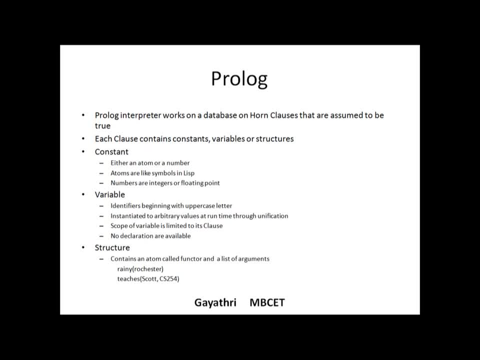 with prologue programming. So prologue is an example of logic programming languages. So this prologue interpreter, it works on a database of Horn classes and all these Horn classes are assumed to be true. So that is the first assumption. it works on the database of. 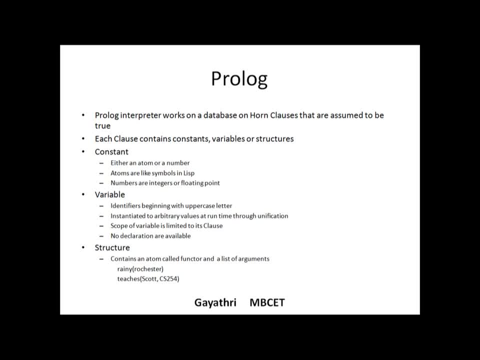 Horn classes and all the Horn classes are assumed to be true. Now each class can contain constant, variable or structure. Now we should know what are all these? So first, constant: what is a constant? A constant can be either an atom or a number. Atom are just symbols in list, Normal symbols in. 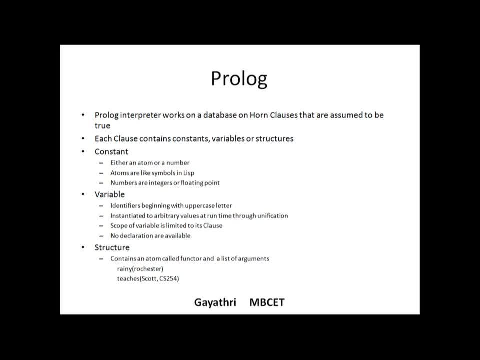 language Numbers. it can be integers or floating point numbers, So constant means it can be either an atom or a number Similarly variable. as we all know, just like in other languages, variables are identifiers beginning with upper case letter. There is no lower case letter, All the. 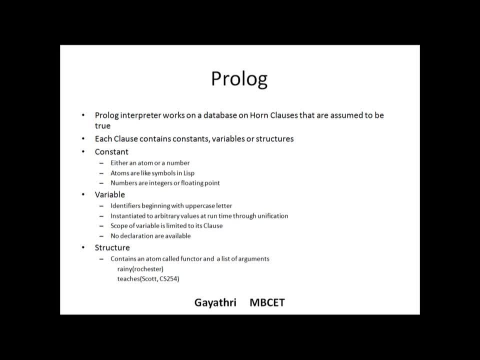 variables in prologue begins with upper case letter, and these variables are instantiated to arbitrary values at runtime through unification, and scope of this variable is limited to its class. No pre-declaration is available. What is a structure? A structure contains an atom called 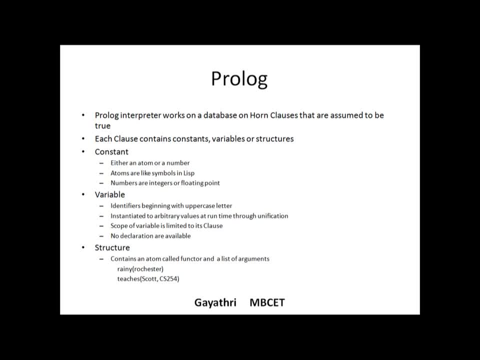 functor and a list of arguments. So atom means it can, sorry. constant means it can be either an atom or a number. Variables are just symbols in list, Normal symbols in list, Normal symbols in list. So variable identifier which begins with the upper case letter: Structure: it contains an atom called. 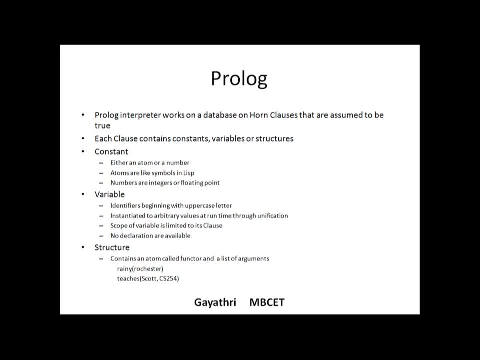 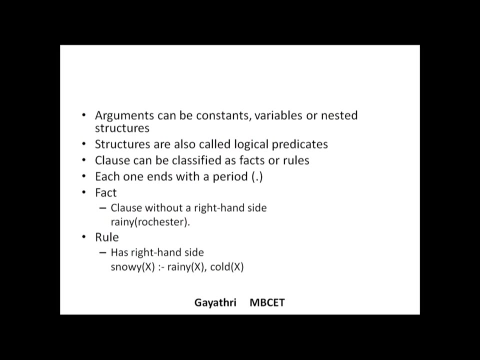 functor followed by a list of arguments. Argument can be 1 or 2 or n, and the number of arguments we call it as arity of this structure. So arguments can be constants, variables or nested structures. Structures are also called as logical predicates. Now this horn class can be: 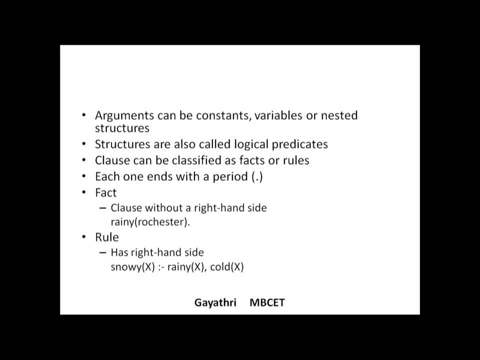 divided into two. One is fact and the other one is rule, and each of these is terminated with a period. operator dot operator, We will define what is a fact. So fact is a clause without a right hand side part. A clause without a right hand side part is called as fact, That is, you won't have. 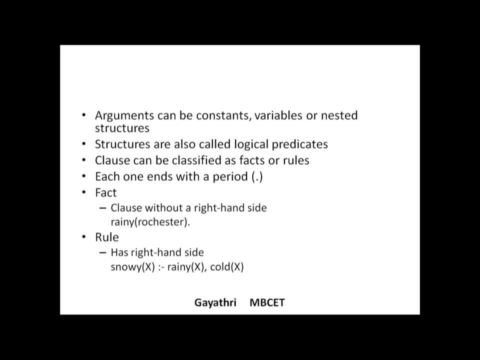 the terms, only the head part will be there. that is fact. Rule means it has the right hand side part. Rule means it has the head. the head of the head is which is left hand side. The other half is called as right hand side as well, so it has the right hand side as well. That is the entire clause can be. 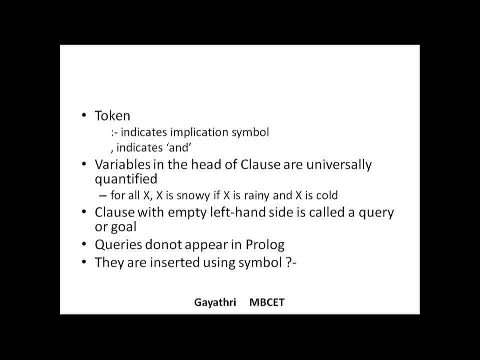 called as rule. So clause without right-hand side is a fact and a clause with right hand side is a rule. This I have already mentioned. what is this token and what is the token Now? variables in the head of the clause are universally quantified. so all the variables in the head are universally quantified. 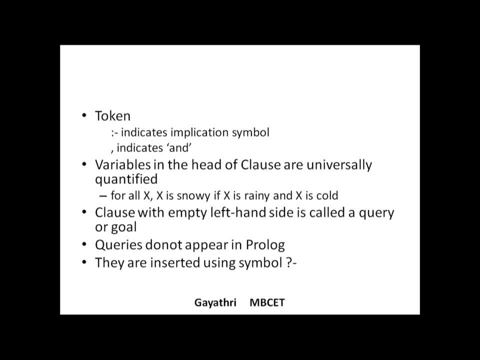 quantified Clause with empty left hand side is called as a query or goal, Empty right hand side is called as fact and clause with empty left hand side is called as query or goal. But this head part will be missing, So queries don't appear in prologue, but we'll insert them when needed. 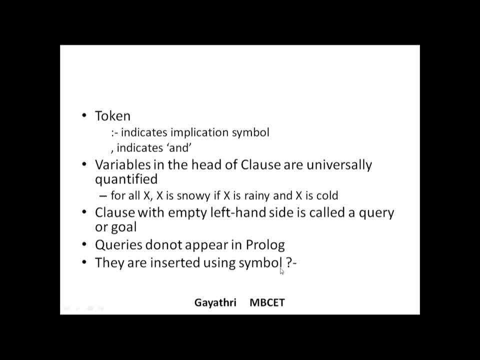 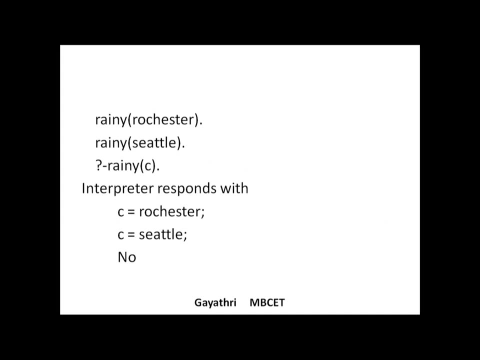 using the symbol, this one question mark and a hyphen. So three definitions. we have seen, which is very, very important fact. then rule and query. So this is the example of fact. Rainy of Rochester. Rainy of Seattle- Now I'm going to query the interpreter. Rainy of C. Look at here. C is a. 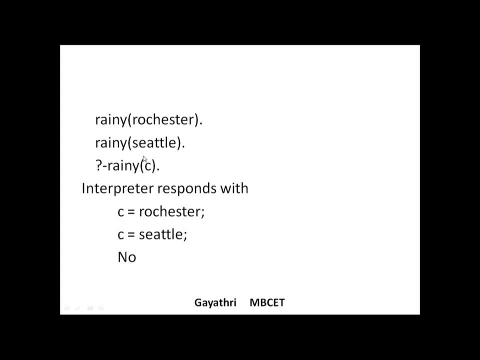 variable. So what the interpreter will do is it will perform the unification. First value of C will be Rochester. When I give a semicolon it means that continue. So it will further search the database to match the value of C. Again, there is a matching, so it will return Seattle. I give a semicolon again. so 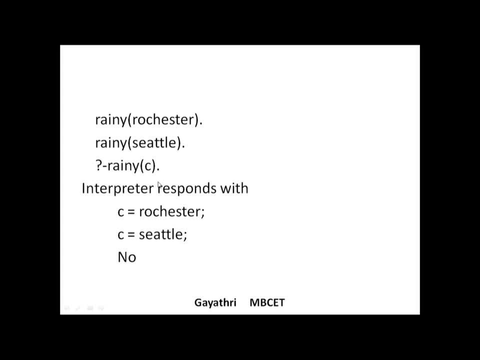 it will go to the database and search for a matching value. Since no more matching value is there, it returns a no. So similarly, you can see here I have given a set of facts and rules. Rainy of Seattle. Rainy of Rochester. Cold of Rochester. 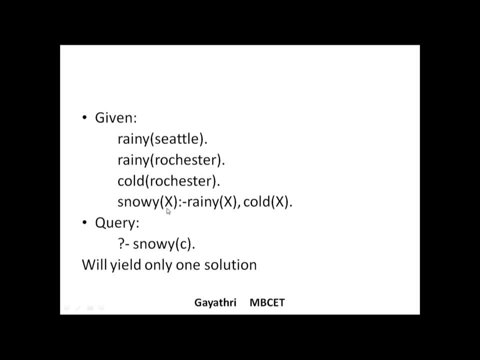 So these are facts and this is a rule. Snowy of X, Rainy of X and cold of X implies Snowy of X. The query is: Snowy of C. Now, see, here is a variable. See, here is a variable So. 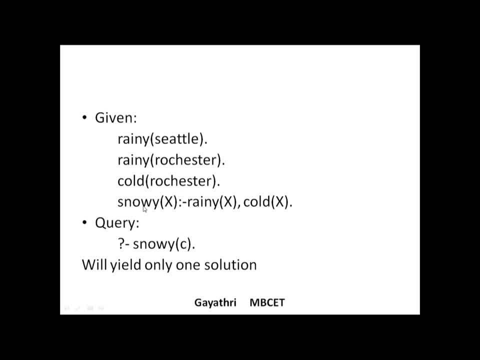 what it will do is it will search in the database. So in the database it has something like this, It has a rule like this. so what it implies is it will check. it will check if it can unify this x okay with some value. so it will check. uh, rainy of x, rainy of seattle, rainy of rochester is there? 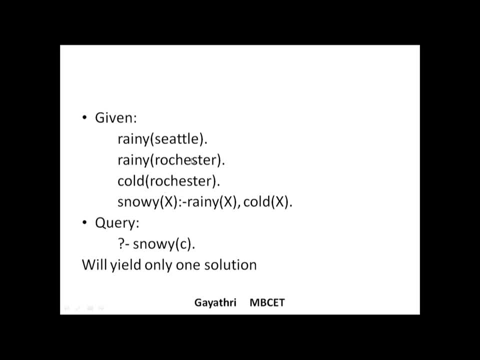 cold of x matches with cold of rochester, so since these two are matching, so the value of x will be taken as c. sorry rochester, and now it will take us rainy of rochester, and rain cold of rochester implies snowy of rochester, so c will be mapped with rochester and this will snowy of. c will yield.